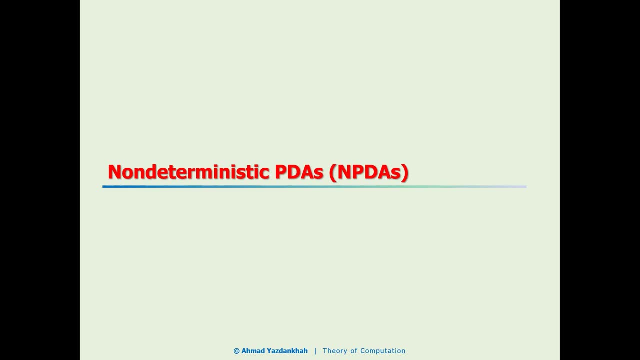 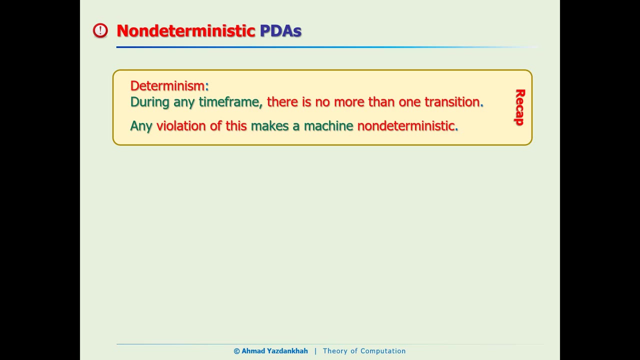 we want to focus on the non deterministic PDAs. let's start with the determinism definition. to refresh your mind. you remember that we said: during any time frame, there is no more than one transition. this is the definition of the determinism. so it means that there should be either zero transition or one. 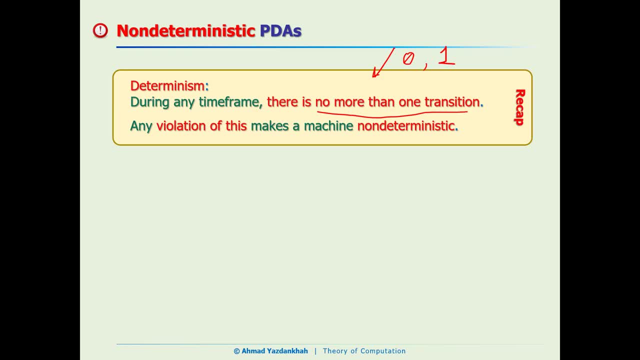 if there are more than one transition, it means that it will be a violation of the definition of determinism, and that makes the machine a non deterministic. so now the question is how this definition will be violated. we have two different way to violate this determinism: either the lambda transition or 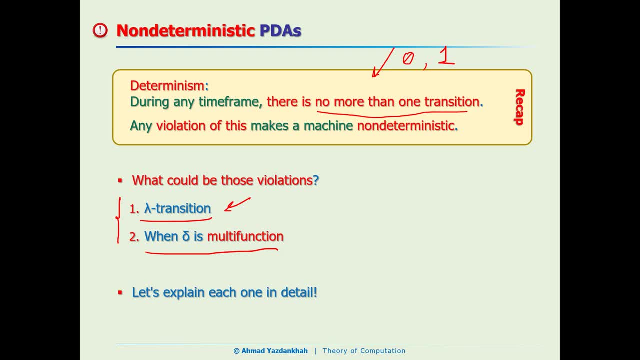 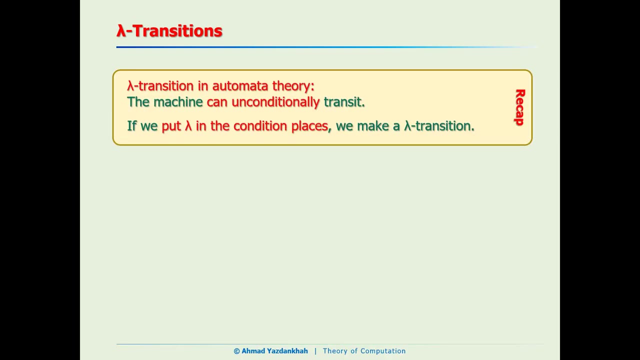 multi function or multi valued function. okay, so let's start with the lambda transition. to refresh your mind, let's review what was the lambda transition. lambda transition in any kind of automata it means that machine can unconditionally transit. so it means that if we neutralize the 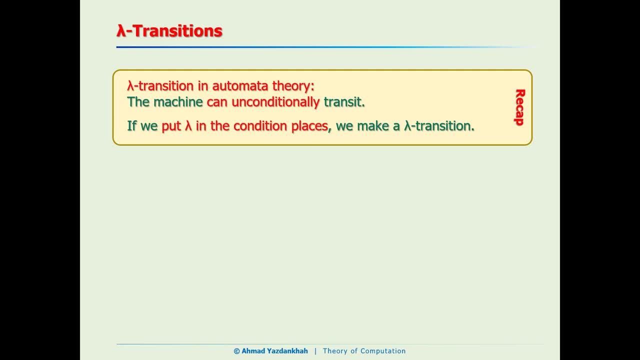 condition for transition. if the machine can transit unconditionally, how can we do that? here is what we did in the DFS and in a phase. so we put the input symbol as the lambda. but PDA now has two conditions for transition: input symbol and also the top of the stack. so we need to put lambda in. 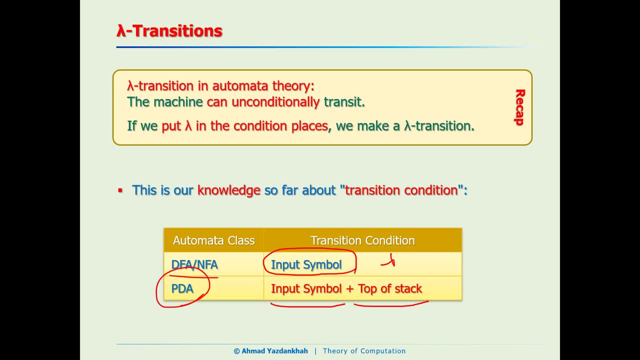 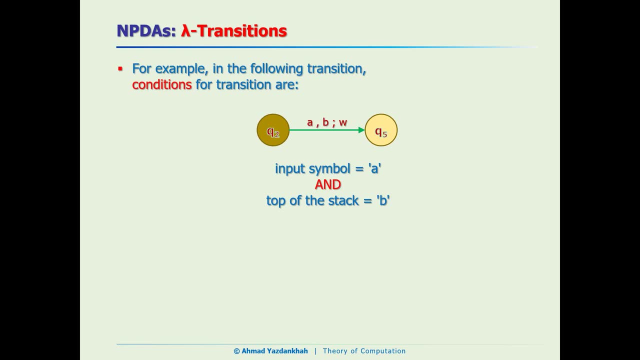 both of them to make a lambda transition. what does it mean? yeah, let's look at this example. so we have a and B. this guy is coming from the input symbol, this guy is the top of the stack, so both of them are condition for transition. we need to put lambda on both of them. so how? this way? right, but even though this, 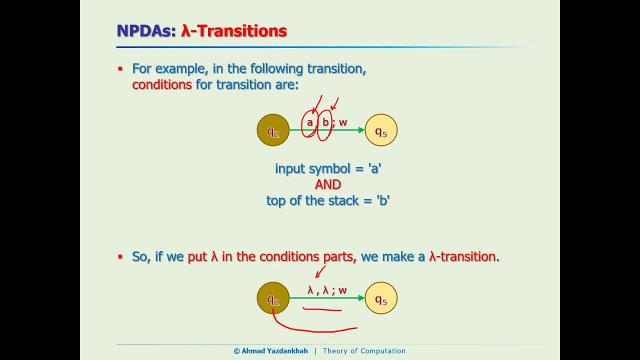 guy is coming from the input symbol. we need to put lambda on both of them. so how this way? right, but machine unconditionally can moves from q2 to q5. but it needs to do something right, it needs to push. this ww is string, whatever we put it here, right? okay, so theoretically this is a lambda transition. 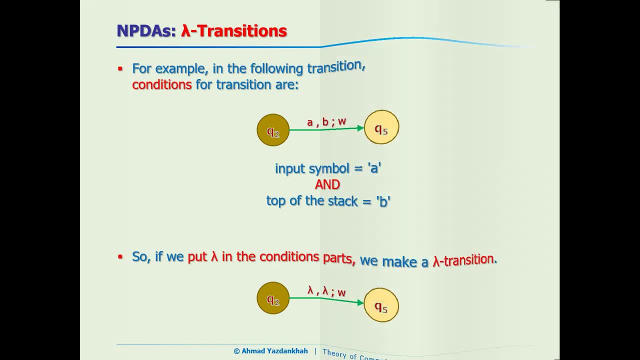 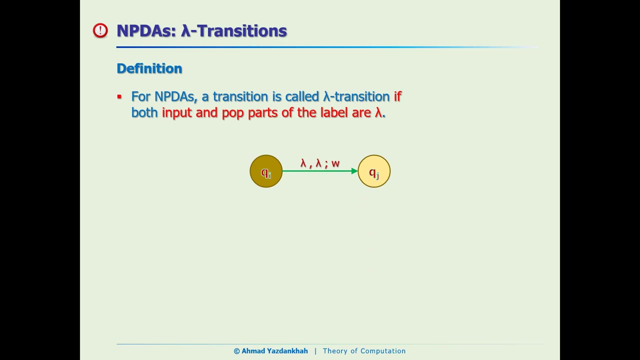 but in practice, really, it makes the design more complex. right, and I I will explain that we need to a little bit simpler. but before that, what is the lambda transition in PDAs? yeah, just putting lambda in the input and the pop part. so this is the lambda transition. okay, so in practice, as I explained, we 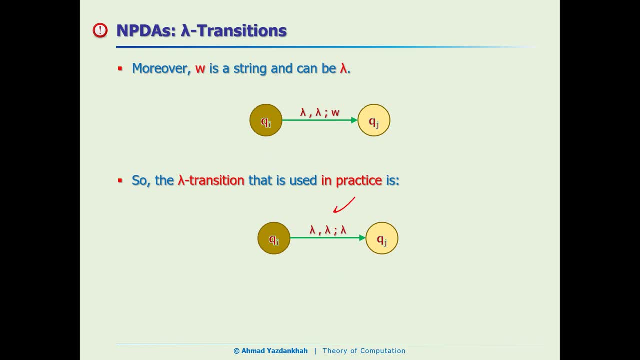 will be using this guy that is lambda, in all of those three parts and in this case, machine unconditionally moves from the qi to qj and it doesn't need any. you know pushing as well. okay, now let's talk about the multi-function example. so this is another way that we violate the determinism. 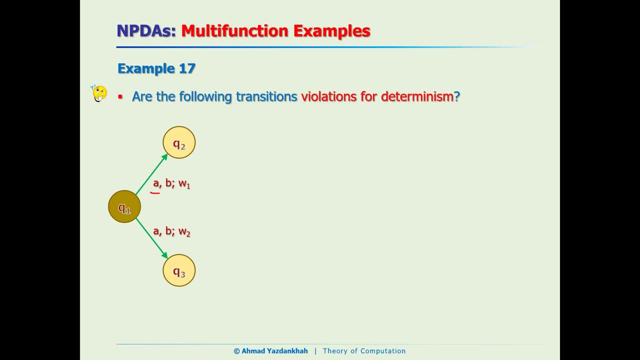 look at this: if the input is a and the top of the stack is B, move to q2 and push w1, but wait a minute with exactly the same conditions, right? so this is one simple example that it's a violation of the determinism. so I ask this question: is this a violation? yes, definitely it is, because machine 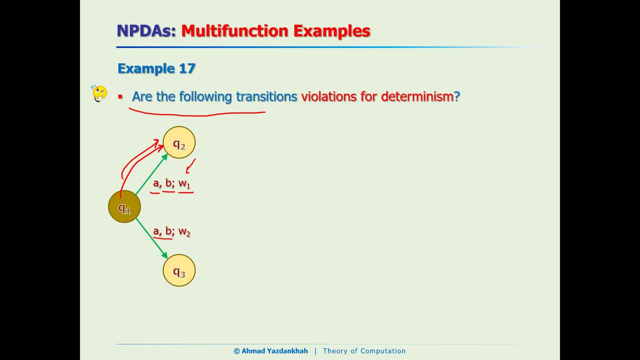 can move to q2 and push w1 in the stack and at the same time machine can goes to q3 but push something right. so to handle this situation, definitely machine needs two processes, right? definitely this is a violation of the determinism. I put together some other examples to show you that. 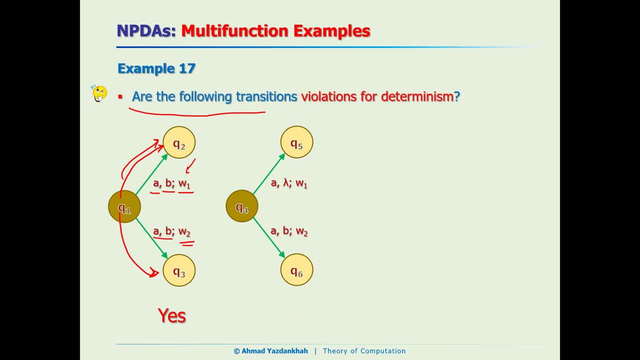 how different situation can happen. look at this one. this guy is saying that if the input is a and the top of the stack is B, go this way. but this guy is is a little bit different. it is saying: if the input is a, don't care about the top of this tag. so when machine encounters these two guys, then 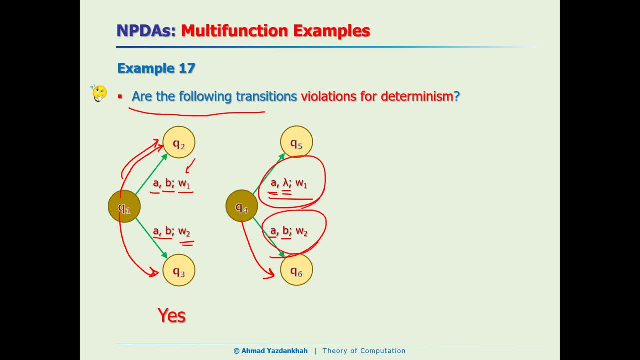 it has both of them satisfied, right? so machine can goes to q5 and also, at the same time, machine can goes to q6. so definitely this is another violation. we have more examples. look at this one in this way. we are saying that don't care about the input symbol, just check the top of the stack. 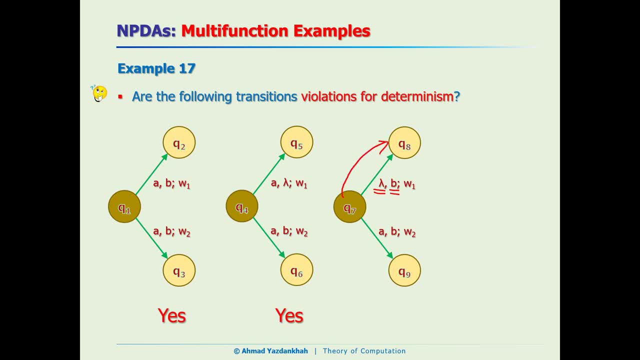 if it is B, move to q8 and push w1. but this guy is saying the same thing, right? it is saying that if the top of the stack is B, yeah, exactly like this one. and if the input is a right, if really the input is a. on the 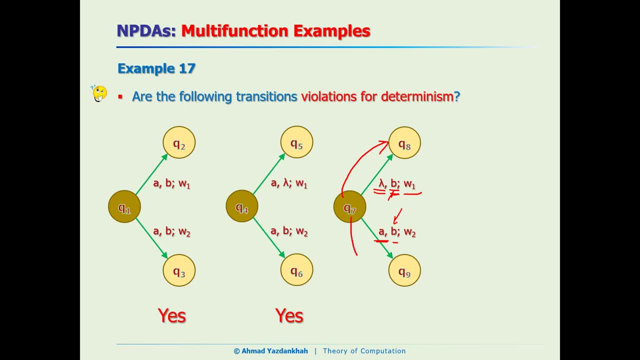 tape, then machine can moves to here and also machine can move here, so we have two possible transition at the same time. so definitely this is another violation of the determinism and another example. here we are saying that this is actually a lambda transition machine unconditionally can move here and push w1, but 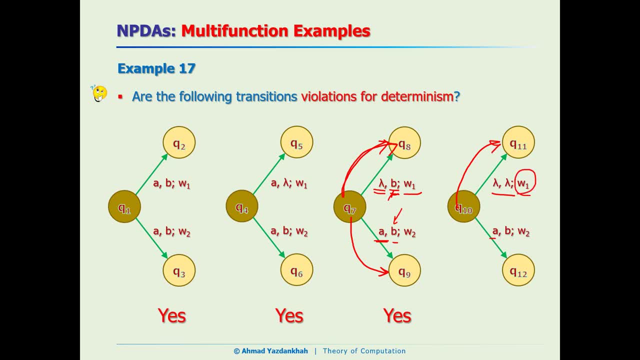 ______ and push w2, but the takeaway is that it is a very, very weak one. but in this case, if W1 into the stack, but here we have the input symbol A and top of the stack is B. so in this case, I mean, if really the input symbol is A and if the top of the stack is B, then both of these. 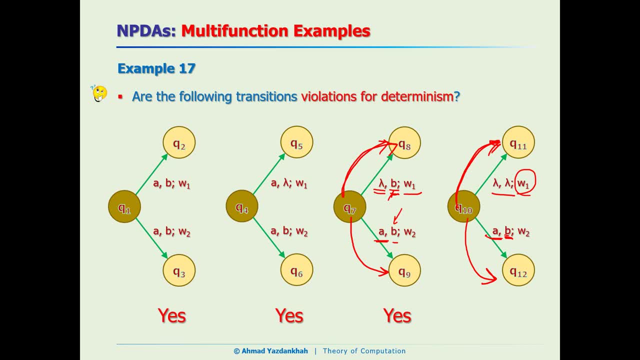 transitions are possible and this is another violation of the determinism. so it means that in some situation, all of these four are violation of the determinism. we have more situation. how about this one? this guy is saying that the input is a, top of the stack is B, but this is input a, but 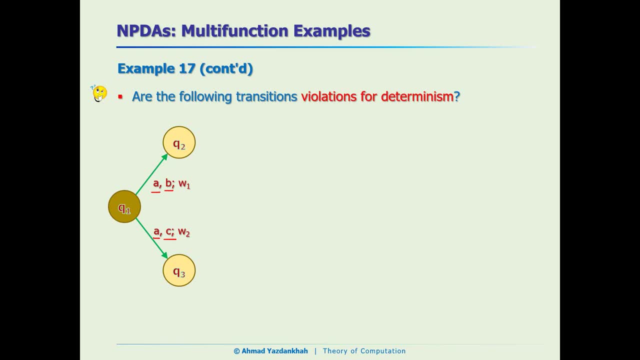 the top of the sexy. so definitely is not a violation. how about this one? this one is again not a violation because the input symbol is different. yeah, with these examples I want to show down both of these conditions should be the same, somehow, right? in those cases, then definitely there will be a. 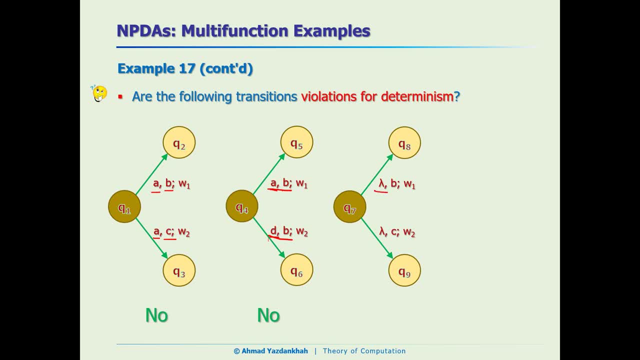 violation of determinism. how about this one? don't care about the input, top of this stack is B. go to q8. yeah, don't care about the input, top of the stack is B. go to B and which is in a random order. and here it is. why is that the two? 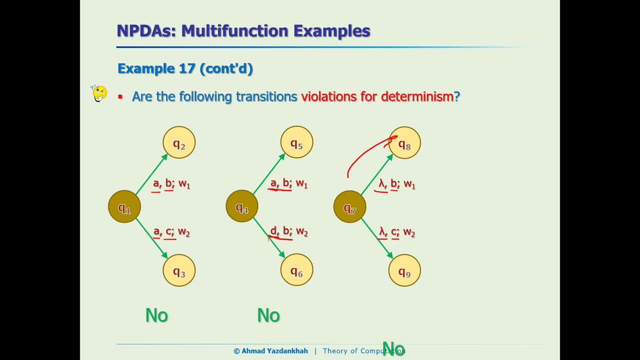 stack is c? yeah, definitely, it's not a violation. how about this one? yeah, this one is no violation. yeah, you can go over that, but we still have more. look at that. so here is it's saying that if the input is a, don't care about the top of the stack, go to q2. how about this one? 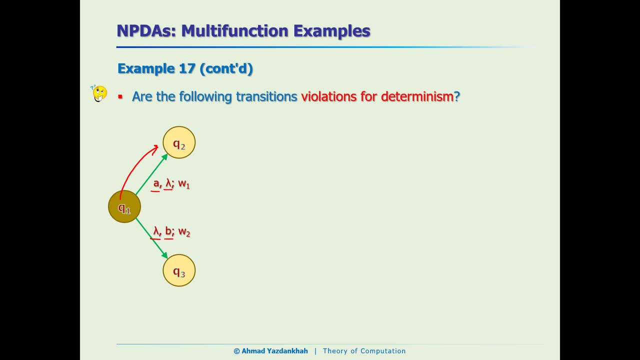 don't care about the input, the top of the stack is b, then move to q3. so if the input tape really is a and if the top of the stack- let's say, for example, yeah if we put z here, and let's say we are here if the top of the stack is b, in this situation definitely this. 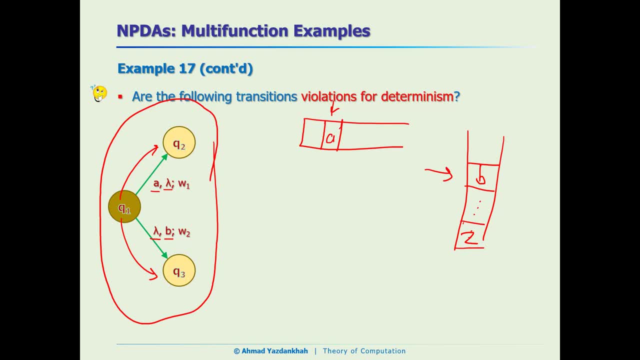 transition will be a violation of the determinism. yeah, i mean in exactly this situation, machine goes to q2 and at the same time it can go to the q3, right? so definitely this is a violation of determinism. we have more here. you can go ahead and try to understand why all of these are violation. 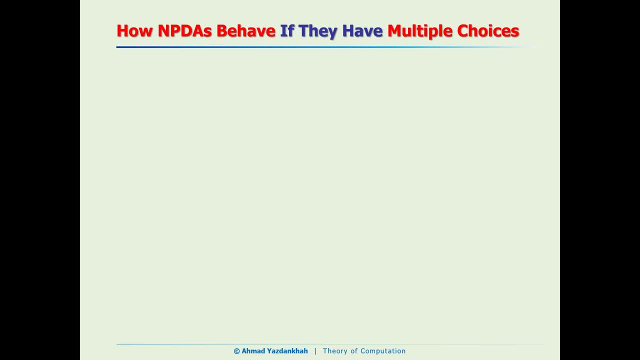 of the determinism. now we are familiar with the lambda transition. also we are familiar with the multi-function or multi-valued functions. now the question is how npdas behave if they have multiple choices. we already are familiar with a very general rule that if machine has several options, it start parallel processing. 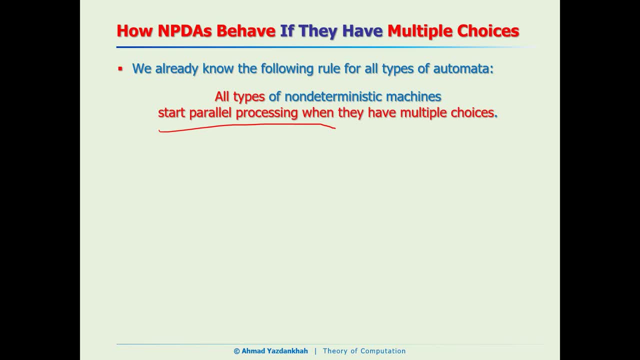 and this is the same rule which is, uh, you know, valid for the npdas as well. so, if you want to be very precise, then we would say, hey, if we have multiple choices machine, start creating new processes, and that creating new processes is exactly the same as nfa. right, i will explain. 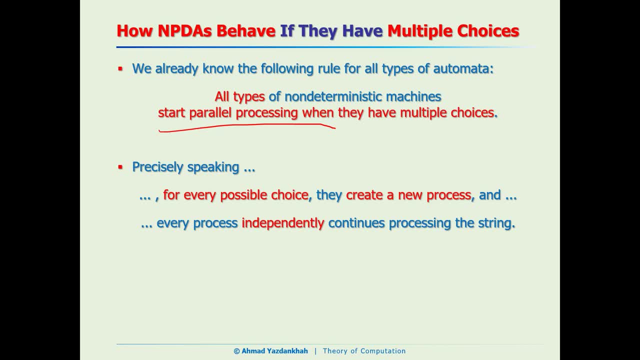 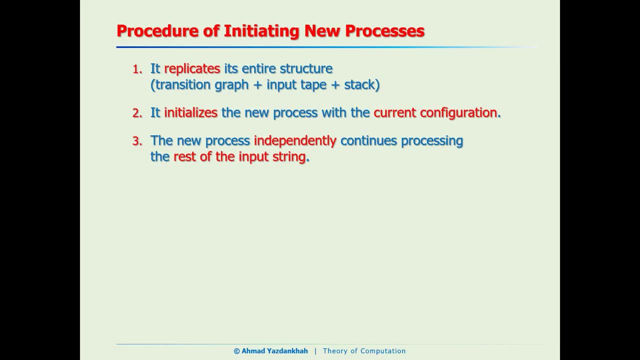 that in a few minutes. but yeah, every process is different. every process is different. every process is start, you know, processing the string independently. okay, now the question is how very simple. the same as the nfas machine replicates its entire structure machine initialize the new processes with the current configuration and each process. 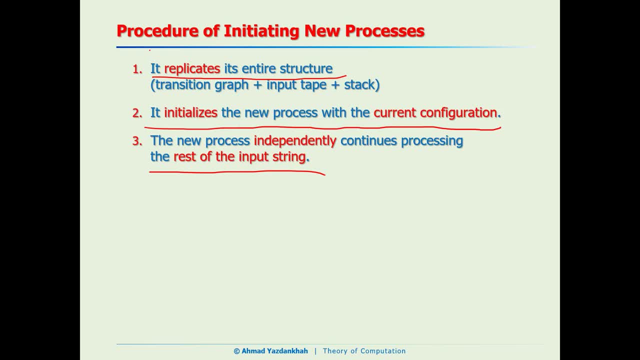 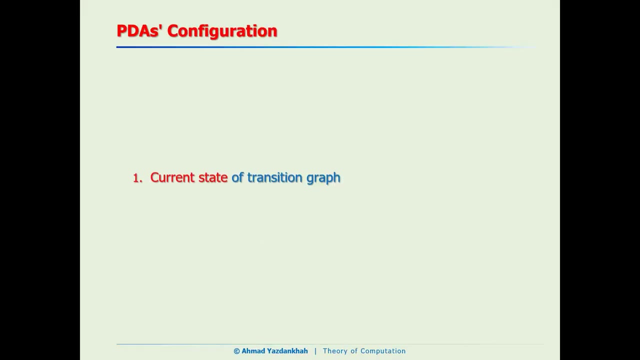 independently continue processing the string. okay, so the only thing that remains to be observed is that the configuration of the npdas and how it is used in the nfa process- in fact, the configuration of the npa process- is common, uh, between the deterministic pdas and non-deterministic pdas, so the current state of the transition graph. 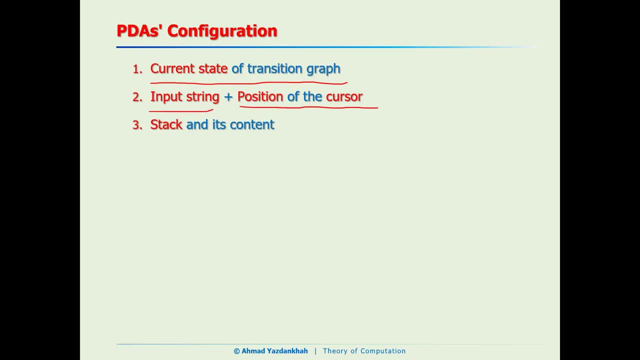 the input string and the position of the cursor, and the stack and its content. so we don't need to talk about the stack condition or the information, etc, etc. just make sure you keep all this in mind. okay, now we are going to talk about the pointer, because it always point to the top of this thing. so these piece of the 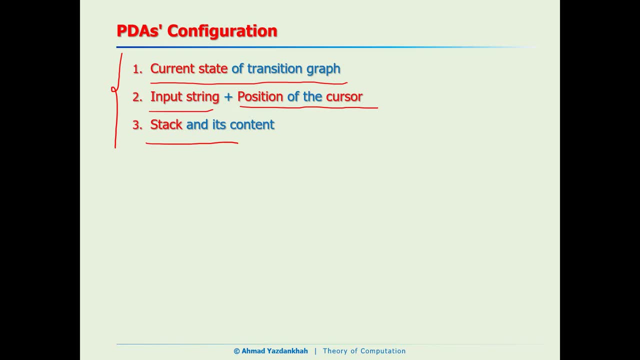 information are the configuration of the PDAs. another question is how, in PDAs, accept or reject the string right. we learned so far that one single process needs to have all of these conditions be satisfied. so halting consuming all of the symbols and halting in an accepting state, right. so this is only for one. 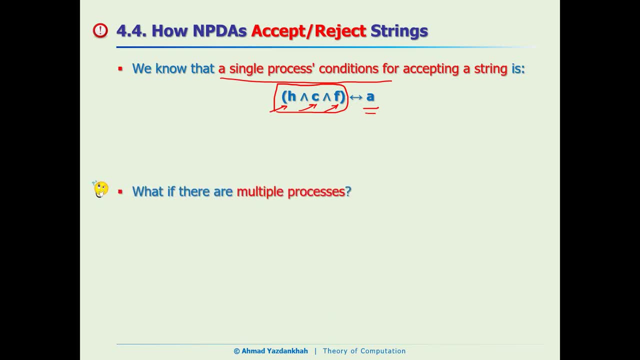 process. but how about if we have multiple processes? yeah, the same rule as the NFAs: if at least one process accept a string, then that string will be accepted. and also for rejection, we need all of the processes reject that you. it's time to turn to the mathematical definition. let's start with the DPDAs. 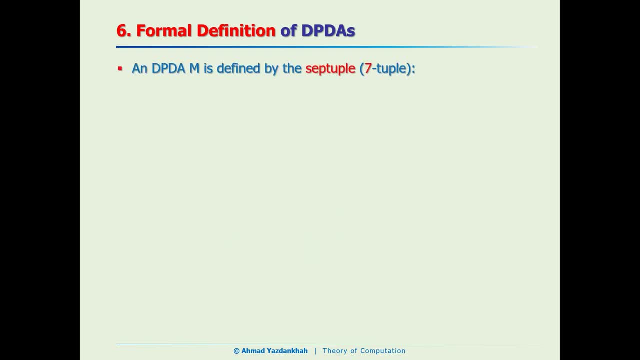 first, a DPDA can be defined by a septuple or seven tuples. so Q, Sigma, Gamma, Delta, q0, capital Z and capital F. what are they? so the Q and the Sigma and the q0 and F are exactly the same as the NFAs, so we are not going to talk about them. let's 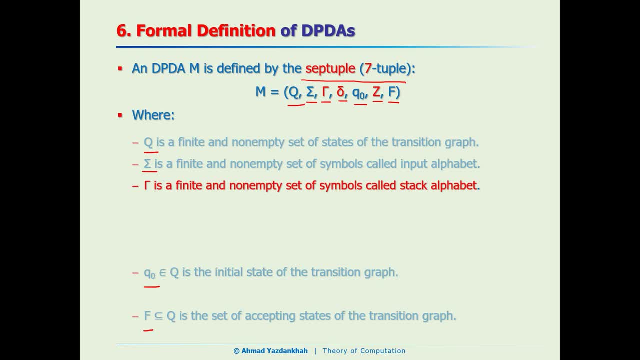 just start with the new ones. the gamma is a finite and non-empty set of symbols called a stack alphabet. you remember I said that a stack alphabet can be totally different than the regular alphabet, the Sigma. yeah, so then we need to specify it with this gray. it can be defined by the direct statement. These are the same two proắper. 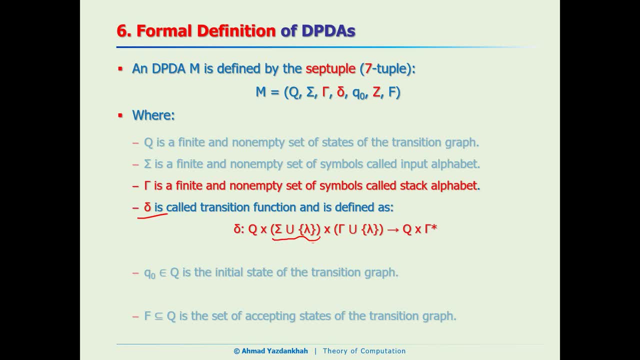 2, So its 0. ,1, 1, 1. 0.. 0.. 1.. 2. ,1. 1. 0.. 1. the gamma with the lambda and then at Cartesian product, between these three and on the range side. 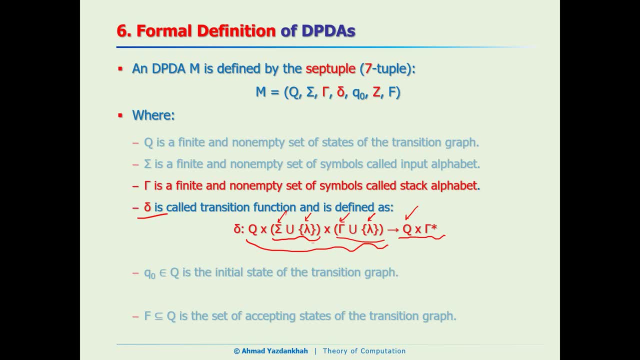 we have Q partition product with the gamma star. what is this? I need to explain that in detail in the next slides, but for now let's accept that, whatever it is right, the next question is: is this a partial or total function? so far, all of them were total function, but this one can be also. 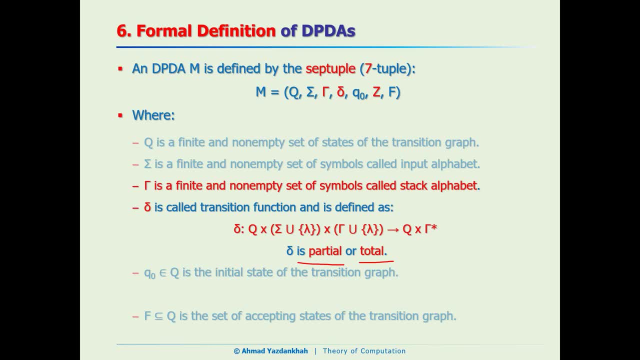 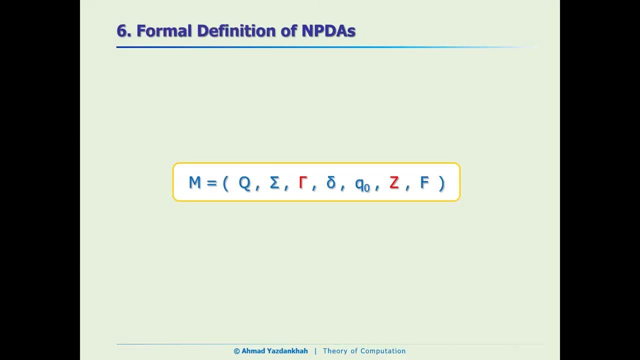 partial function. all right, how about the Z? yeah, Z is part of the gamma, so always, gamma contains the capital Z, because it's an alphabet of the stack on the bottom of the stack and it is a special symbol that we call it stack start symbol. okay, so yeah, just let's have a quick review what is? 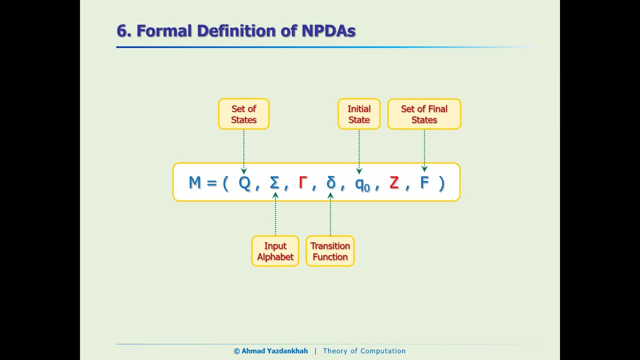 the Q and what is the Sigma? what is the Delta? what is the Q, 0 and F? and these two guys are you the new guys, right? so the gamma is a stack alphabet and the Z is the special symbol for the stack. with that we call it stack start symbol. okay, so now to explain that how that Delta works, let's. 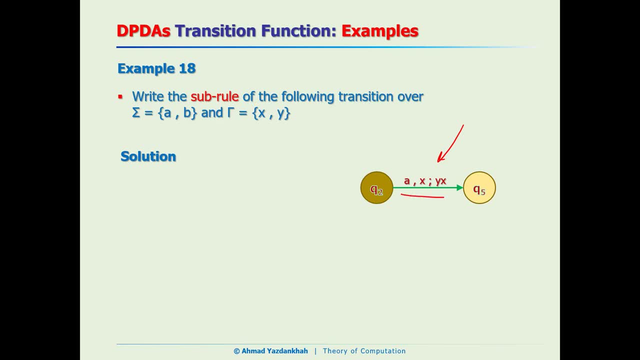 start with this simple example. look at this. the question is: what is the sub rule for this? yeah, we are looking for the delta and what is the sub rule for this? yeah, we are looking for the delta and the and we are looking for theイ right, which is the total weight of. what is the total weight of the? 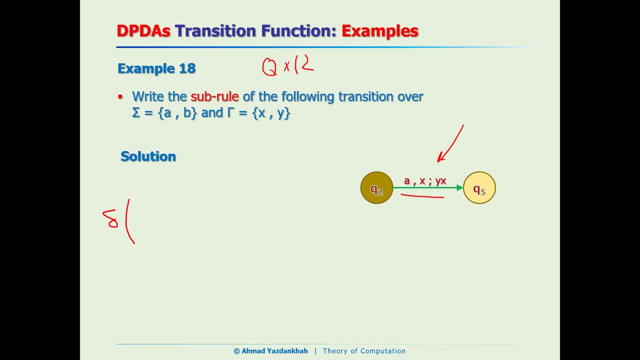 the total weight of this- and we have the total weight- is equal to the volume of identity of in this equation. so we have here delta of the D January, the coordinate in this equation. as this condition, we need to compute the constant loop value in terms of this condition. as this condition, we need to compute the constant loop value in terms of. 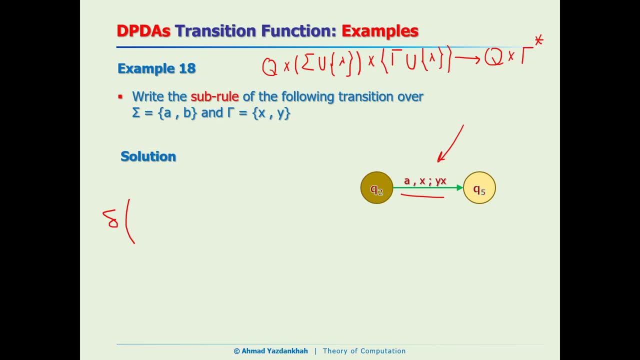 the, but has only one set alpha and minus the dot 해代 the item a件番ne less than oneован given多少 from MA in these with the debate, so no problem. gamma star. so what is this and how can we use that? so in the domain side we have a three tuple. 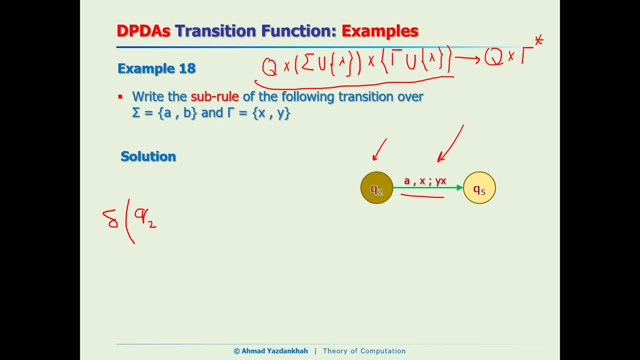 one is q, which is the starting state of the transition, and then we have the input symbol coming from here. so it's coming from here and it will be a, and also we are. we have the top of the stack. it's coming from here, so it is the delta of q, 2 comma a comma, x, then equal to what we need one. 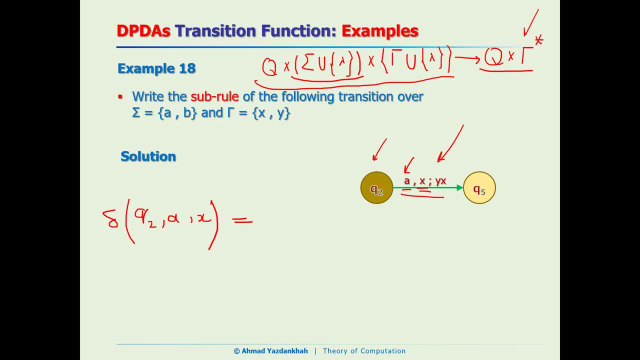 q and one string from the gamma star, right. so it means that go to q5 and push whatever. this is y, x, right. but since we don't have such thing in mathematics, we need to put it somewhere. so we create a two tuple or order pair to show that what the range is. okay, now let me ask this question. 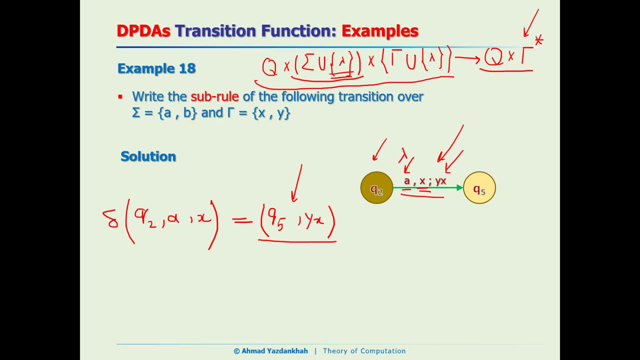 why do we need this lambda? because we can put lambda here, right, and since lambda is not part of the alphabet, we need to union that. how about these guys? so we need to union that. how about this guy? the same thing. we can put lambda here as well. 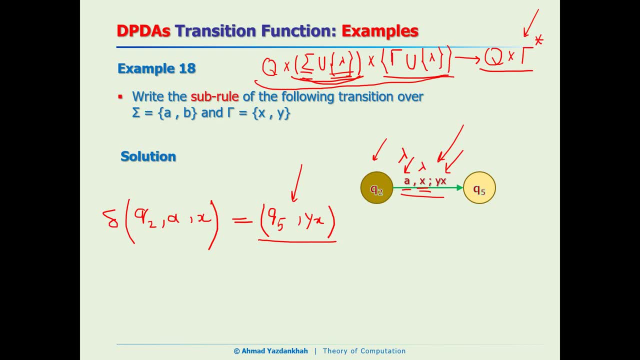 and lambda cannot be part of the gamma, right? so that's why we need to union that, all right. so this is the answer and this is why we had to union the lambda with this guy and this guy. okay, now the question is: how about delta of q2? 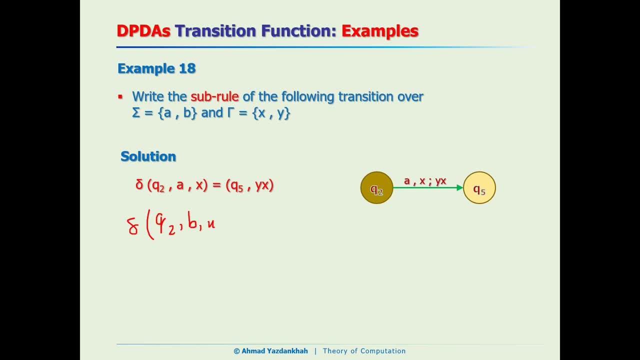 and cancels out b and x. what is the answer here? it is dependent on the equation of q2 of this servicio. cancels out b or x for the da value du. so the appearance here is two gems: dark colored redish and the first one. and then i'm gonna go ahead and screaming. 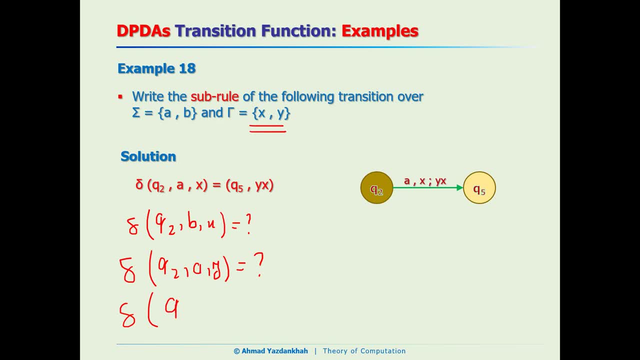 here as well, right, and it's kind of like if you could give you a perfect example. let's say x10, and so the warm up here, let's say큼 cancels out q2 and b and x, and cancels out q2 and b and x, and cancels out b and x, and then 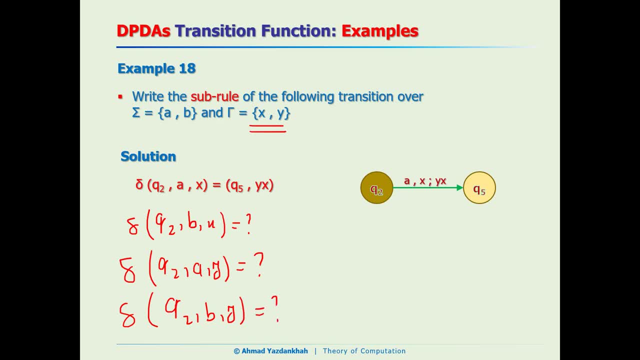 what are these values here? yeah, we don't have any outgoing for all of these three, so actually none of these three. so it means that all of them will be undefined. that's why we said the delta can be partial function, because we have some situation that they are undefined. so, as you see, PDAs don't. 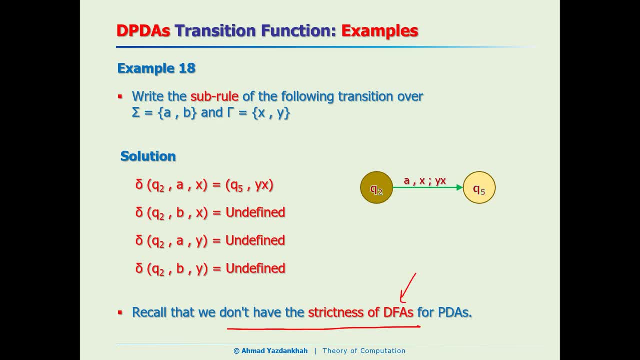 have the strictness of the DFA's, so there are some situations that there is no outgoing for some of the symbols of their alphabet. another question: how can we write the Delta here? so here, if we are in q2 and if the input is lambda? as you see, this is one reason that we put lambda here and 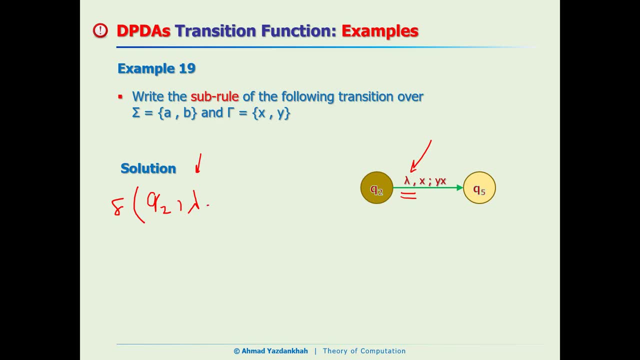 we needed to add it to the alphabet, and if the top of the stack is X, then go to q5 and push Y X. now let me ask a very important question: is this sub rule equivalent to these two? so could we remove this and instead of this one sub rule? 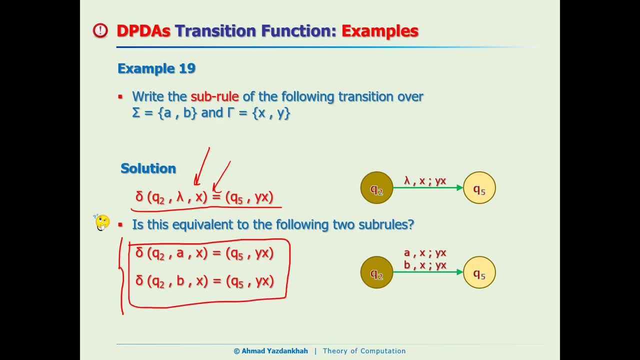 could we put these two? in other words, we consider this lambda as a wild card and we could say: okay, if it is a and the top of the stack is X, go to q5 and push the Y- X. if input symbol is B and the top of this stack is x, then do the same thing. vote for other. 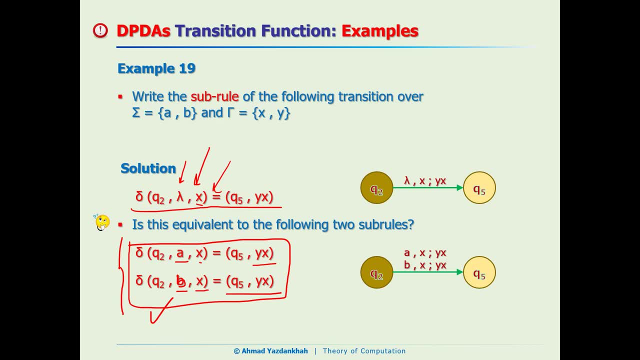 did same thing. you thought we replace the two guys with this one. ok, so you can pause the video to answer the questions. can we can stop the video too? definitely not. they are not equivalent, because if you replace these two guys with this one, it means that if a in the input symbol, then E should be consumed. if A the input symbol, then he should be consumed. 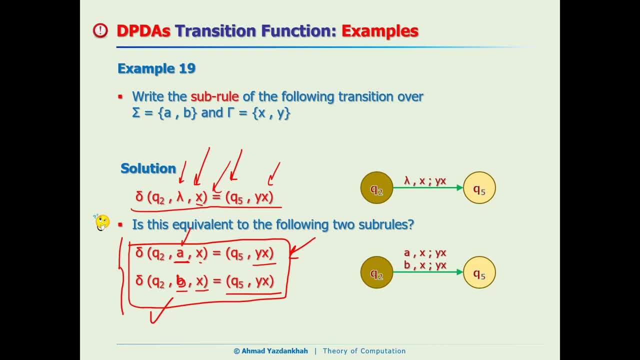 ok, so if A input symbol, then he should. a should be consumed, the same thing for the B. but if we put lambda here, nothing will be consumed. so these two sub rules are not equivalent to this one because of the, the consumption stuff. another example: yeah, this time we put lambda here on the top of the stack. yeah, with the same reason we can say that. 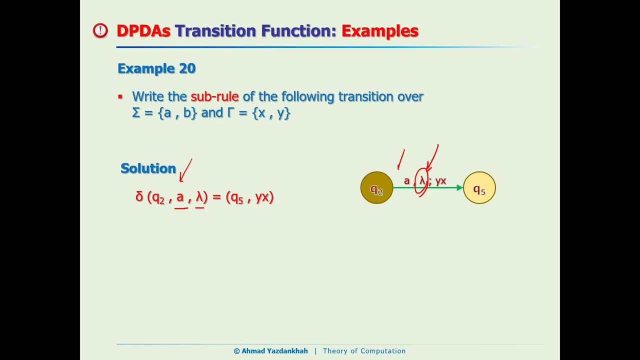 yeah, the input is a and the stack don't care about the top of the stack and the result will be q5 and pushing this yx again. I want to ask this question that can we replace these two guys with this one? for the same reason they are not equivalent, because if we put this guy and this guy 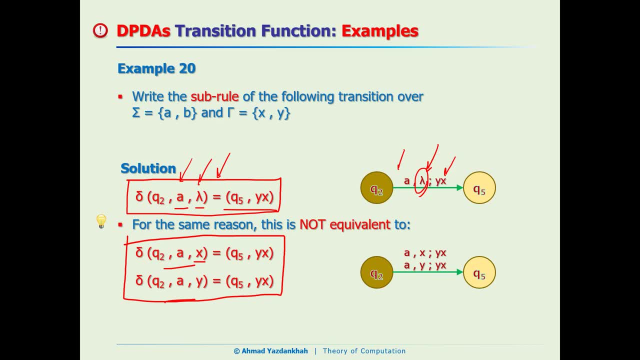 instead of this, then we need to pop something right, but here we don't touch the stack at all. another example: yeah, I think your knowledge is enough for this one and we don't need to talk more about this. the only difference is that we don't push anything. so, in other words, we notice that we can have lambda in. 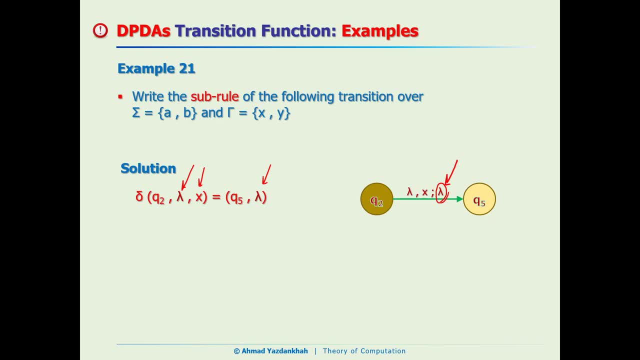 any position here. and the reason that we union lambda with the Sigma and gamma is now obvious. how about the other side? yeah, I mean the pushing this. yeah, we don't need to add any lambda over there, because, if you remember, the range was Cartesian product between Q and the gamma star, and gamma star is exactly like the. 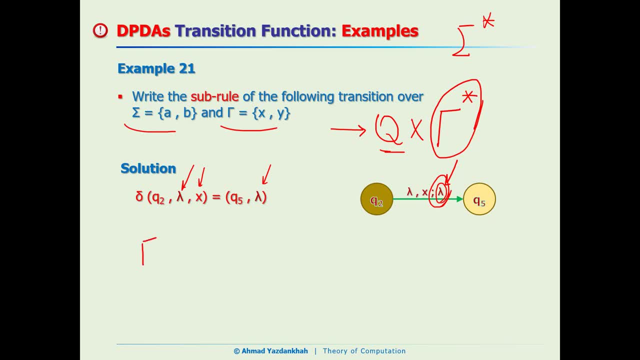 sigma y, Y, point Y and the value of the white square when the gamma goes southまず, in whatever square you want to say, but I find this Ok. liberal and radical lambda exists here, so we don't need to union the lambda here, right and so forth. 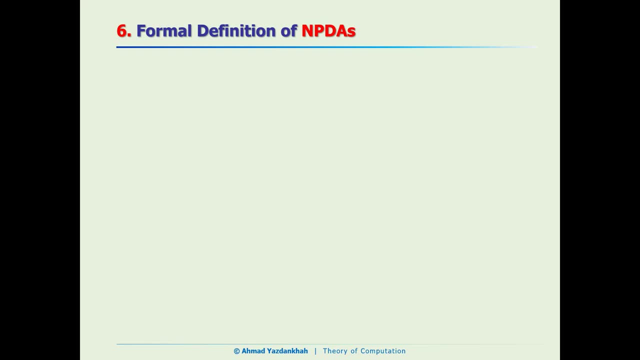 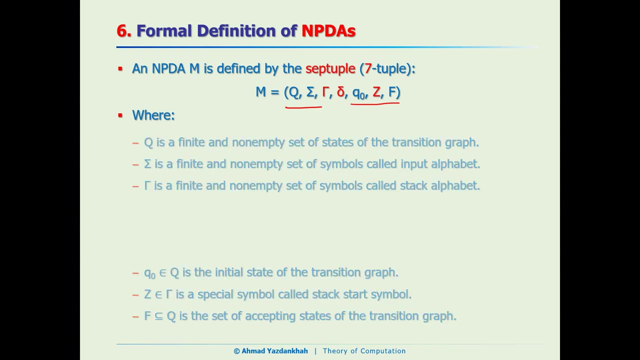 now let's talk about the formal definition of the NPDAs. they can be defined exactly with the sept tuple that we talked for the DPDAs. six of them are exactly the same and we are not gonna talk about them. the only difference will be delta function or transition function. 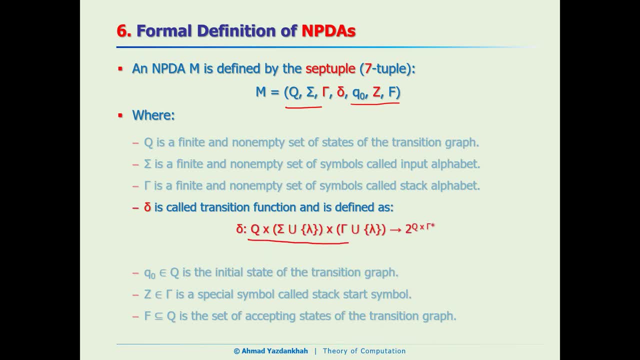 that looks like this. so on the domain side, we have no difference, but on the range side, as you see, we are using the power set. right and why we need to use the power set? the same reason that we talked on the NFAs. we have some situations that we have zero. 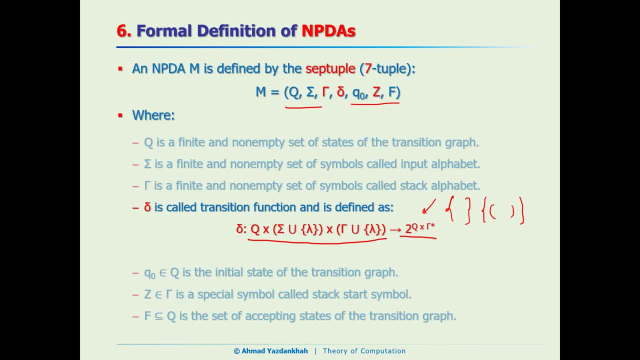 value, or one value or multiple values. that's why we need to put them in in a set right. that's why we are using this power set right on the DPDA. we just had Q cross product with the gamma star. now we are using the same set but the power set for them. 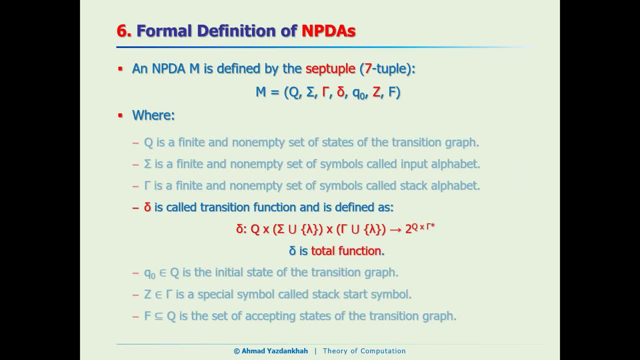 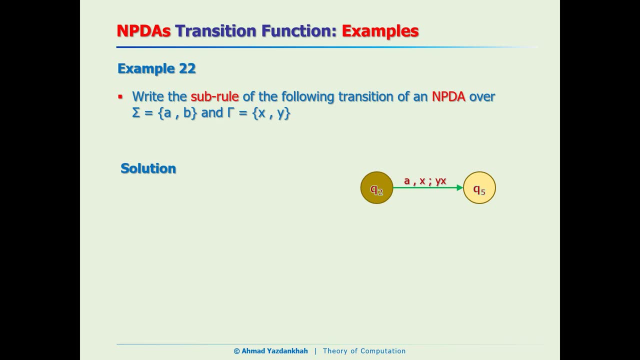 okay, so for the same reason, it can be a total function. now let me take some examples for this. yeah, there is no difference with the DPDA. the only difference is that we would need to put the range inside a set, and there are some situations that we have empty sets, like this: 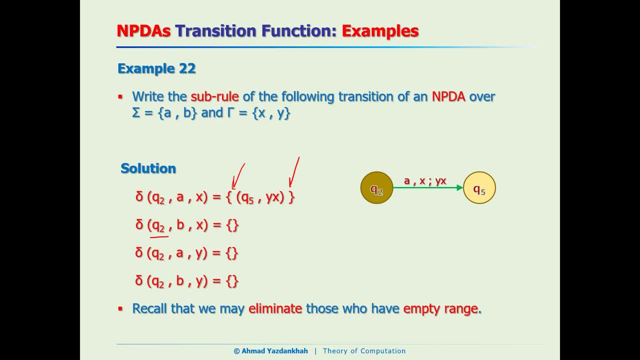 so, since we have no sub rule for the Q2, if the input is b, that's why the result or the range value will be empty, and we have the same thing for the other possible values and, as usual, we can eliminate all of those that are empty and 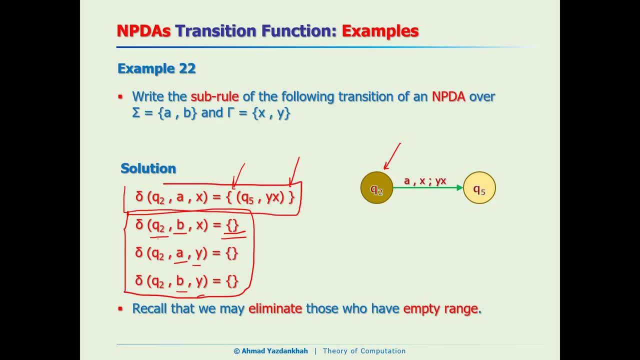 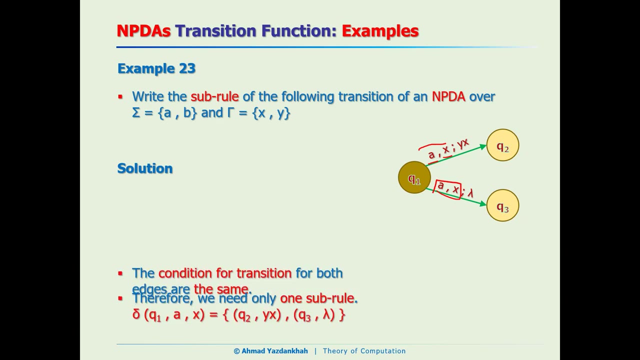 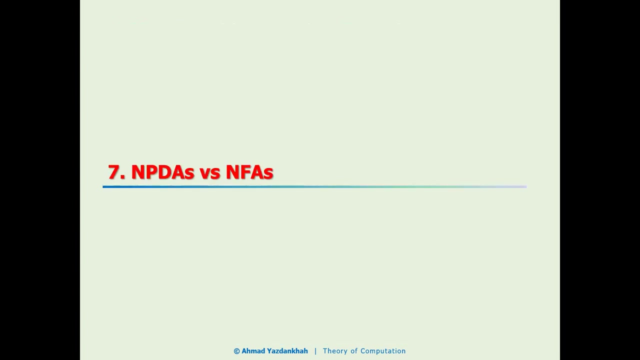 just keep those sub rules. that has some values. another example: here: as you see, the input is a, the top of the stack is x and the same thing here. so in this case we will have two values for the range and we put both of them inside the set. in this section we are going to compare npdas and. 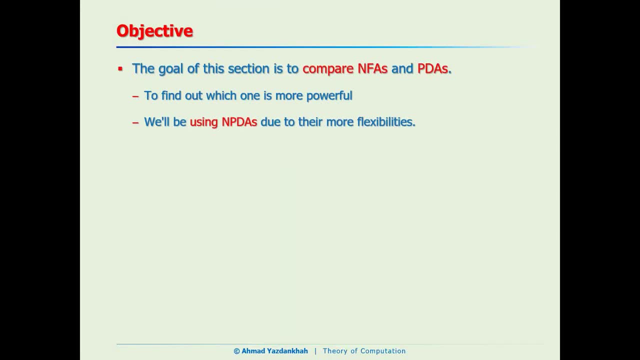 nfas. so we want to know that which one is more powerful. how can we do that? we will be asking two questions when- whether or not, can npdas simulate nfas? can nfas simulate npdas? and the answer to this question shows that which one is more powerful. okay, let's start with the first question. 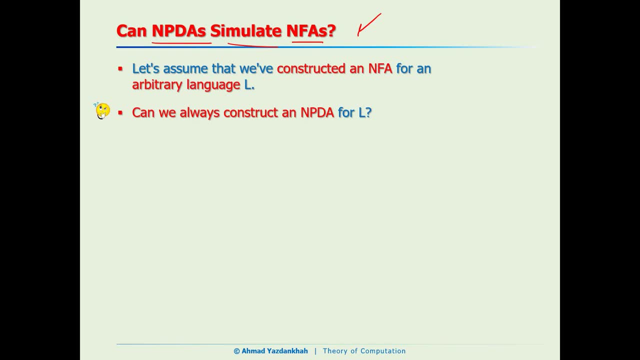 can npdas simulate nfas? what does it mean really? it means that if we construct nfa for a language- so let's say this is a language and we have an nfa for that, right, can we always construct a pda for that pda. when i say it can be npda, it can be dpda, right? can we always do that? if we can do that, 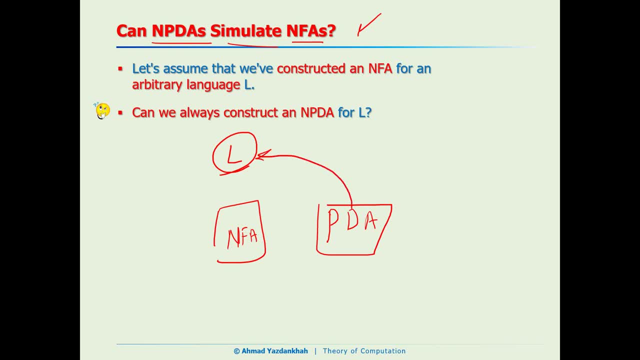 then it means that pda can do whatever the nfa can do, right? so one way is to convert the definition of this nfa to pda. if i can do that, then it means that in fact, with a very simple algorithm, i can convert the definition of nfa to a pda. so in that case, yes, then we answer. 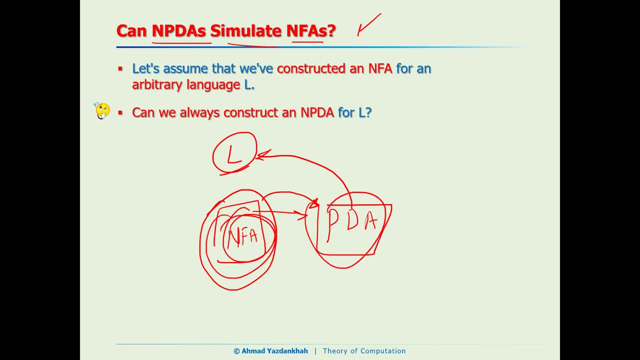 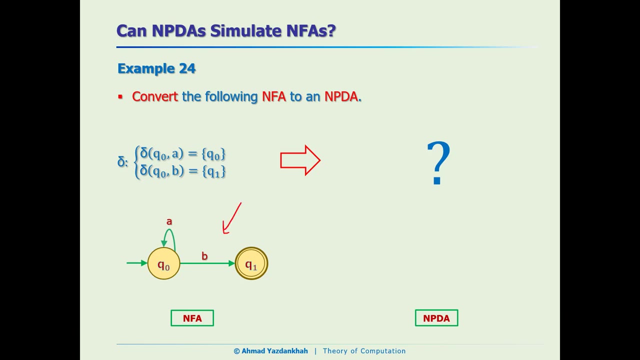 yes, whatever nfa can do, pdas can do as well. okay, how can we convert the definition of nfa to pdas? yeah, let's explain with this simple example. this is an nfa, definitely, and this is the definition. how can i convert this definition to an npda definition? that's a very 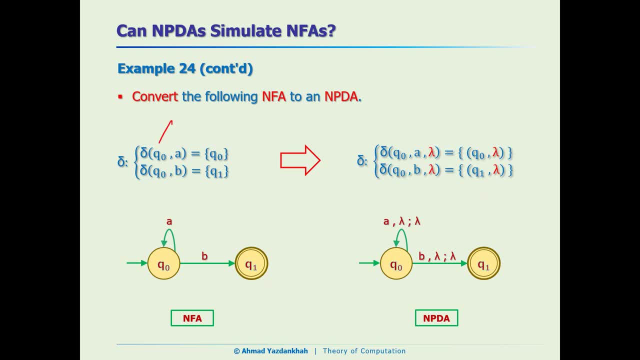 good question here. so look at this delta on the left side and this one. if i just add a comma lambda to this one and put this in an order pair and add a comma lambda here, it will be converted to this machine. will convert it to this machine, right? can i do that? yes, 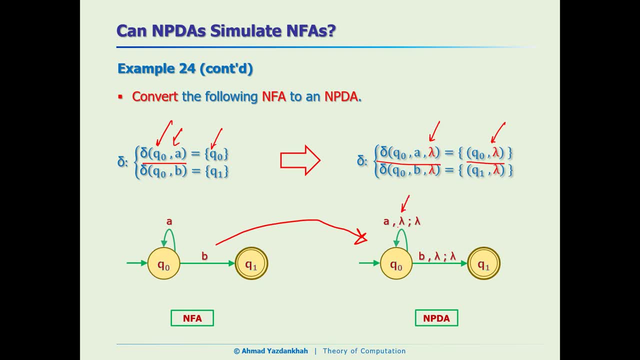 how come? because i am saying that don't care about the top of the stack and don't push anything. so it means that i am trying to not touch the stack at all for all of these transitions. if i do that, it means that i put aside the stack. and if i put aside the stack, what remains? 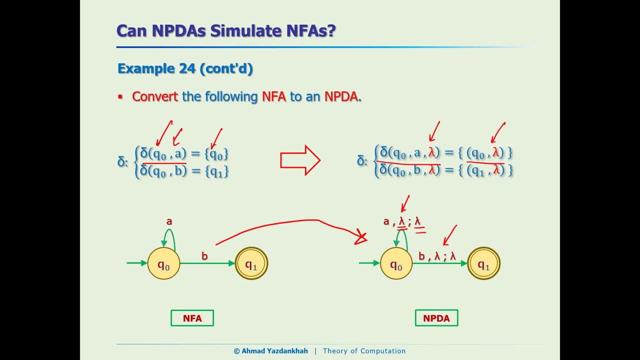 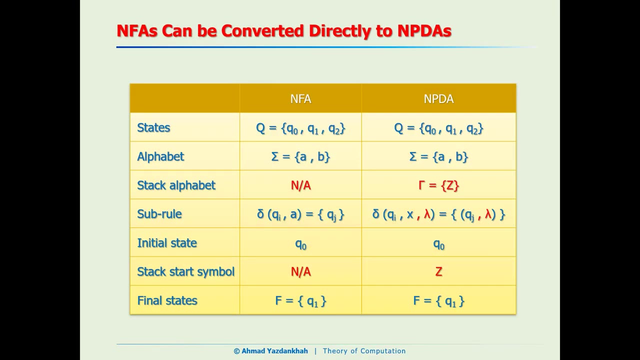 exactly an nfa right, and this is how we convert the definition of the nfas to pdas right. okay, so let me summarize that. is it possible or not? so should we change the states? no, the states is the same thing. the alphabet no changes. a starting symbol for the npdas is z. 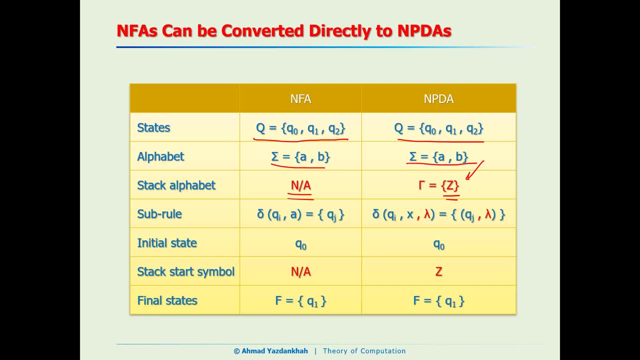 but this guy doesn't have, of course it doesn't have, right. i just need to add this right. no more alphabet for the stack, just the z is enough, and it is always the constant thing. i can add this, right. how about the sub rules? yeah, exactly so just add a comma lambda here and a comma lambda. 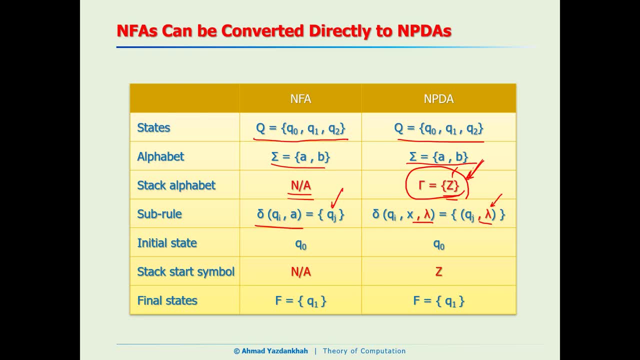 here and put the range instead of this qj. just put it in an order pair. no changes to q0: 0. of course it doesn't have the Z here, we just add it. this is a constant thing. and no changes to the accepting states set right. so you agree that this is a. 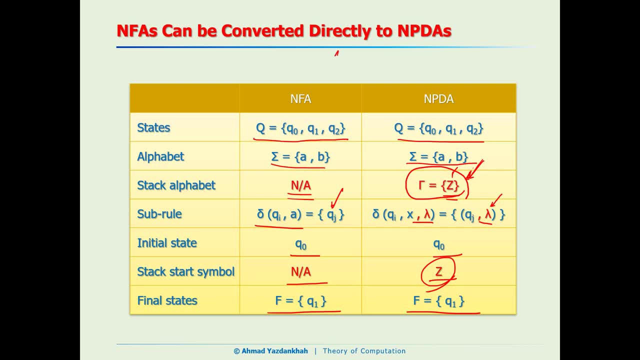 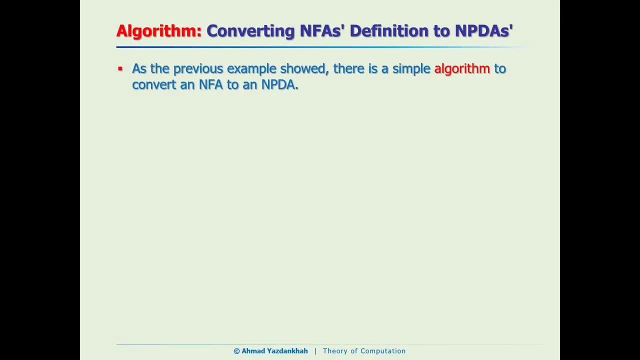 algorithm that we can do on all of the NFAs and convert them to NPDAs. so if this is the case, I can do that. always, right? I put all of those explanation here for your reference. so now we understand that. yes, whatever the NFAs can do, NPDAs can do the same thing. alright, okay, now let's. 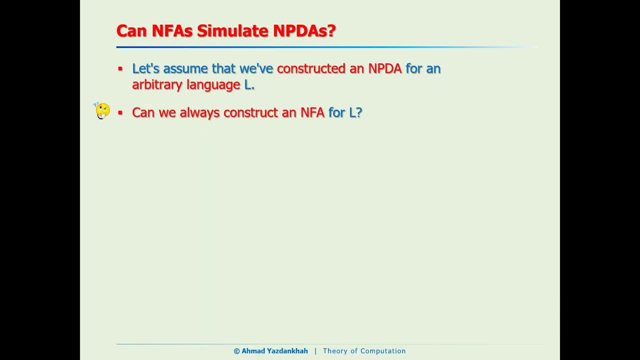 ask the question the other way around: can NFAs simulate NPDAs? if I have a language like and I create an NPDA for that, can I always construct a machine that you know, construct an NFA machine to solve the same problem? obviously no, because at 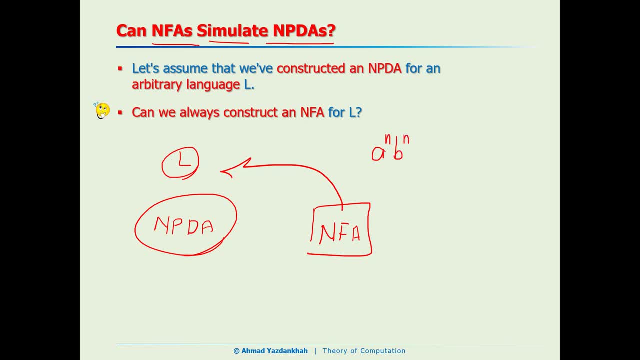 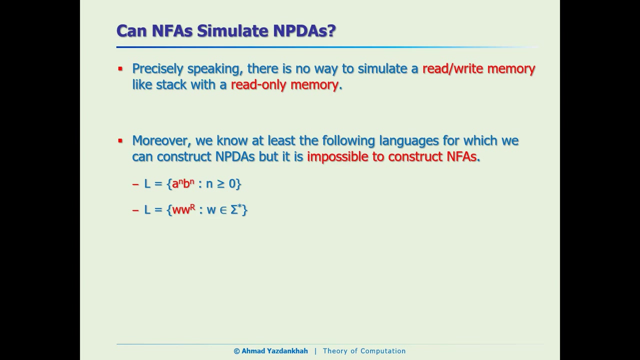 least I know one language- that I couldn't do that for NFAs, but I could solve or recognize them with NPDA. so this is the answer and this is the reason right. so it is really no way that we can simulate the stack operation with the NFAs. that doesn't have any writable memory at all and these two are just. 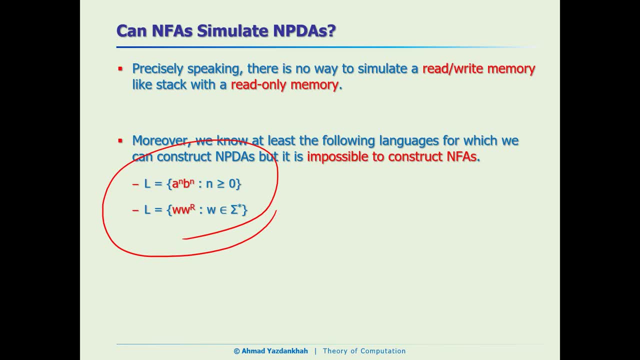 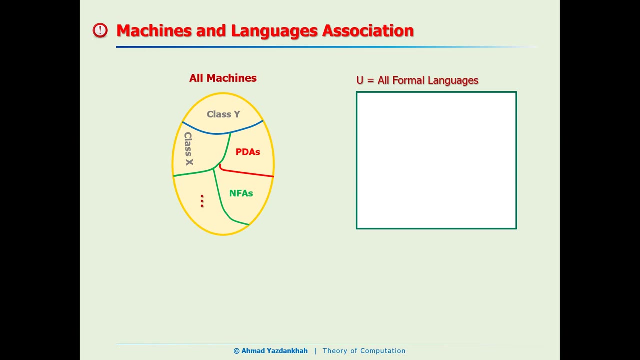 counter examples. that shows that NFAs cannot resolve the same problem or understand these languages, but NPDAs can do that. now question is: what is the next step? let's shine our knowledge and let's look at the machines and languages Association one more time and see what. 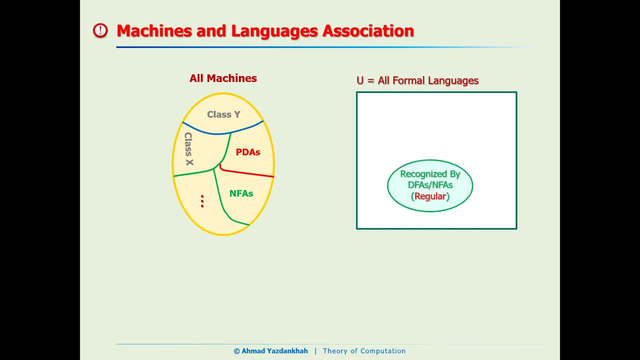 we got so far. so we know that NFAs and DFAs just accept this portion of the languages that we call them regular language, and now we learned that PDAs can accept more than that portion that DFA's and NFA's can understand or recognize. is there any other languages that we cannot? 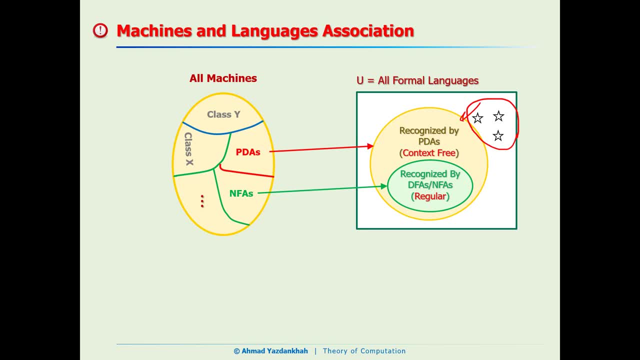 understand with the PDAs. that's something that we need to find out, but before going further, this portion of the languages we learned that we call them regular language, this portion that can be recognized by the PDAs, we call them context free. right, just keep this name in your mind, but we still don't know. 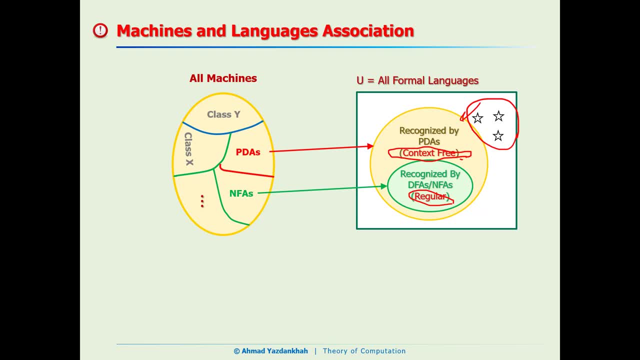 what it means. yeah, we will get back to this context free later, all right, so if this is the case, then definitely PDAs can accept more than that portion that DFA's and NFA's can inside these types of languages. so we can prove somehow that PDAs are more. 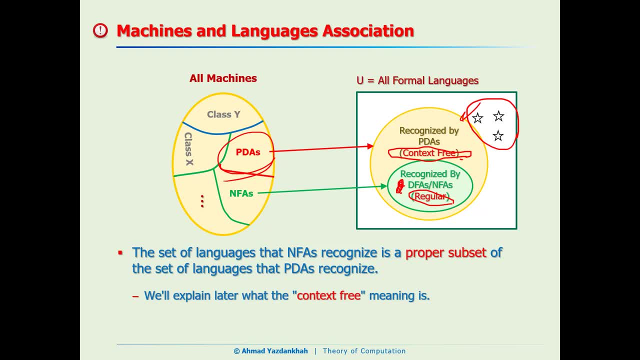 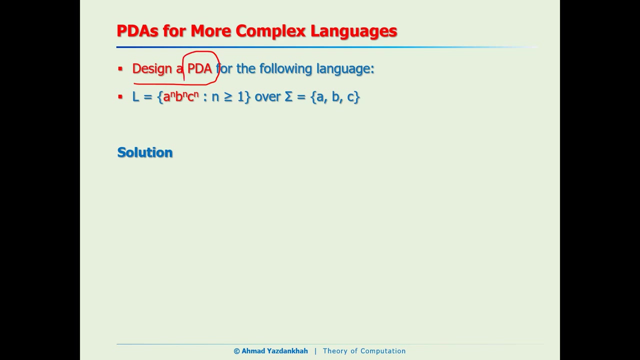 powerful because we prove somehow that all of these languages here can be recognized by the PDAs, but at least there are some languages here that cannot be recognized by the DFA's and NFA's and definitely PDAs are more powerful. okay, now let's pause the video and try to create a PDA. it can be DP da. 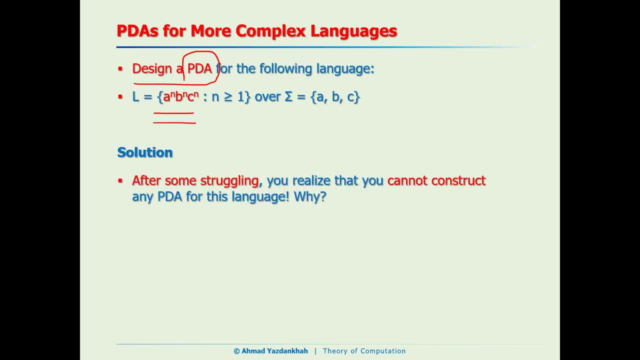 DP da and NP da. for this reason? because if we want to use PDA's and NFA's for this language, yeah, after some struggling, we find out that we cannot do that. and the same thing for the WW. this language can not be recognized by PDAs. so what is the reason? because the stack is not. 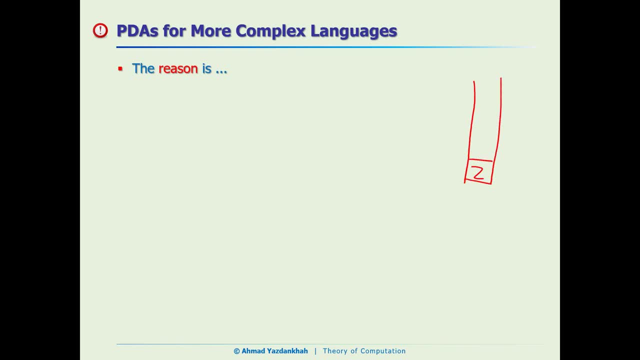 that much flexible. what does it mean? it means that, for example, if you are here, let's say you are here and we have some stuff here, right, if you want to access this information, you need to pop all of these and to reach here. it means that you will lose all of those data. so I want to say that a 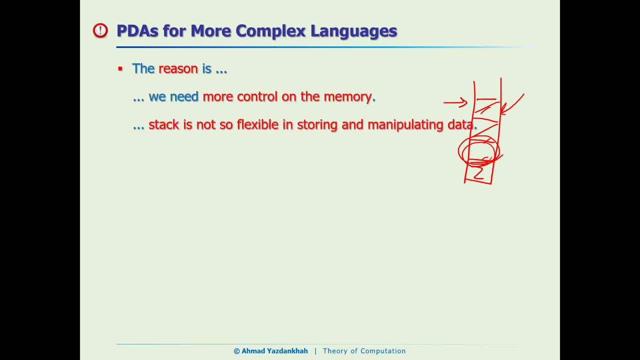 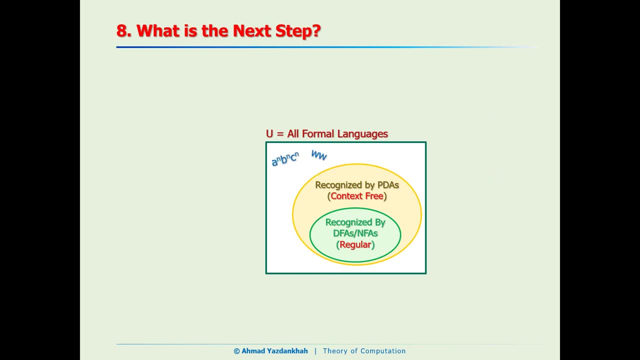 stack is not that much flexible for storing data and manipulating the data. okay, so if this is the case, then we have some languages like this that cannot be accepted by the PDAs. so what is the next step? absolutely, we need to introduce a new class of machines that can at least accept some more languages. 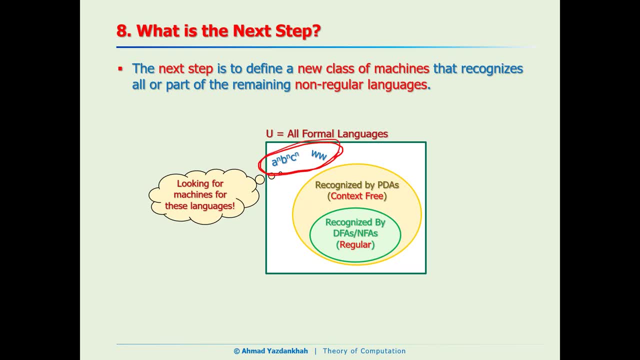 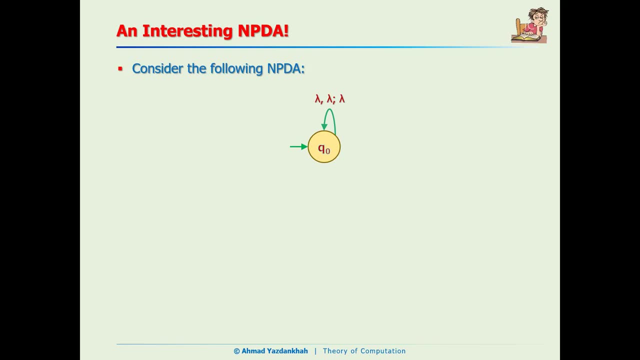 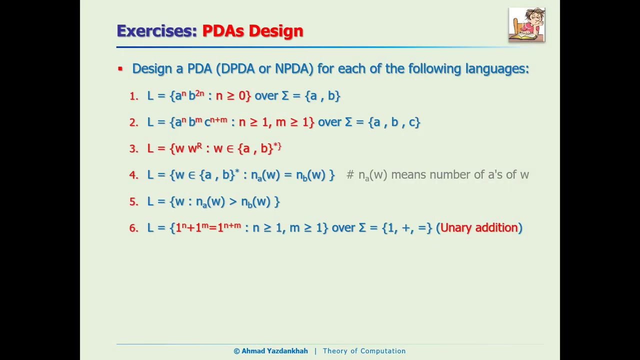 more than the whatever that that the PDA can accept. I put some interesting in PDA for you guys, so try to simulate this with the jflap and try to answer this question. this can be a good exercise for you guys and I put some other exercises here and also another exercise.